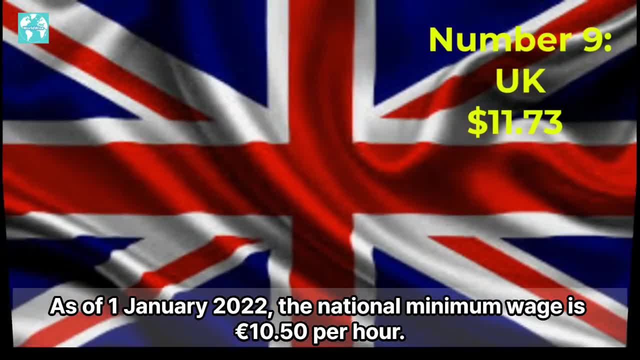 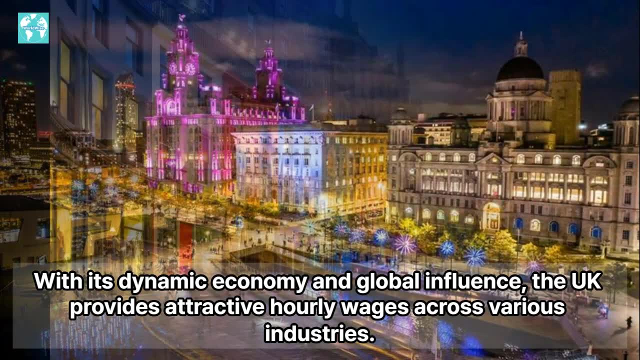 wage is €10.50 per hour. Number 9. UK: With its dynamic economy and global influence, the UK provides attractive hourly wages across various industries. Whether you're in finance, technology, creative arts or professional services, you'll be able to earn a substantial hourly wage. You'll be able to earn a substantial 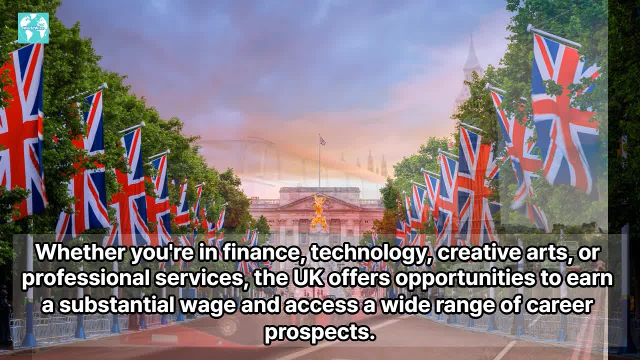 hourly wage. You'll be able to earn a substantial hourly wage. You'll be able to earn a substantial salary. You'll be able to earn a substantial salary. The UK offers opportunities to earn a substantial wage and access a wide range of career prospects. 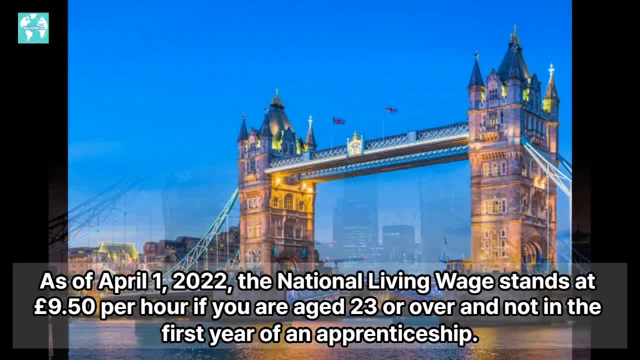 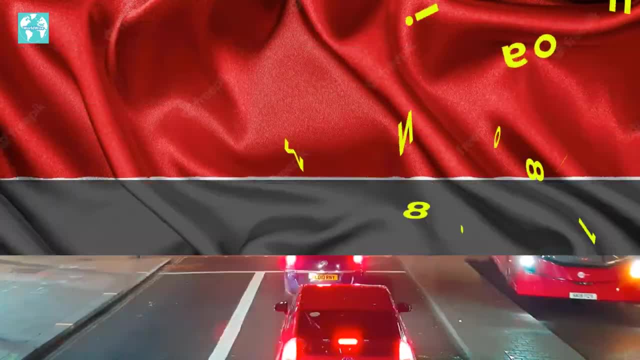 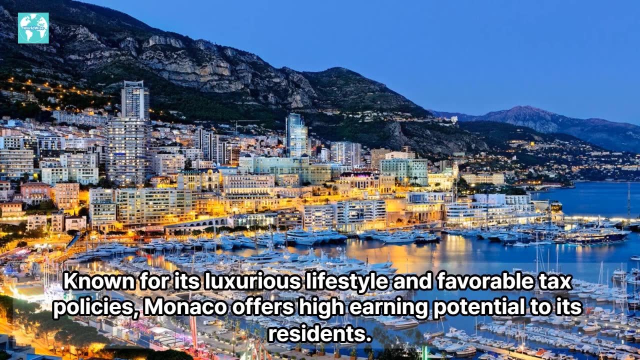 As of 1 April 2022, the national minimum wage stands at £9.50 per hour if you are aged 23 or over and not in the first year of an apprenticeship, A Tie for number 7.. Monaco, Known for its luxurious lifestyle and favourable tax policies. 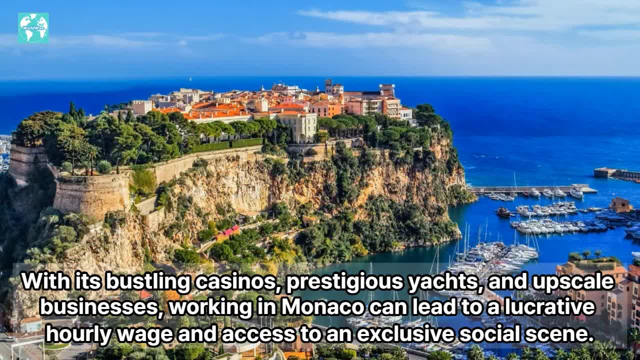 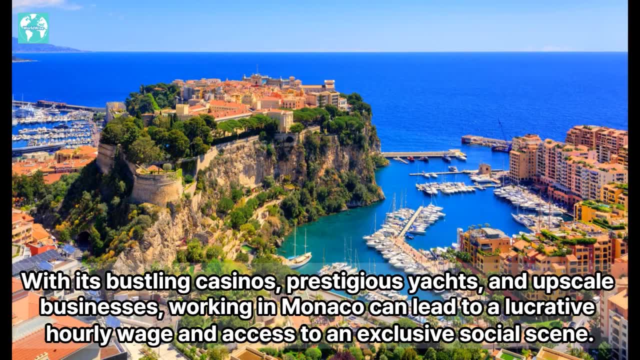 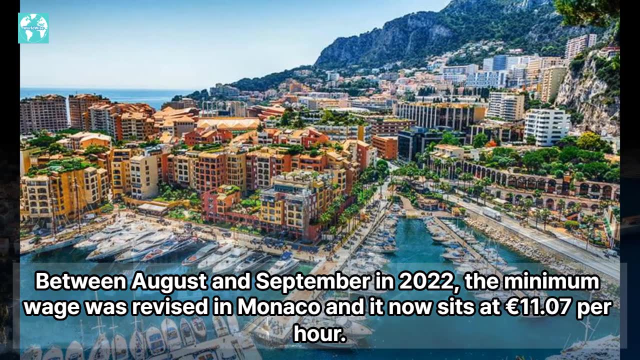 Monaco offers high earning potential to its residents, With its bustling casinos, prestigious yachts and upscale businesses. working in Monaco can lead to a lucrative hourly wage and access to an exclusive social scene Between August and September. in 2022, the minimum wage was revised in Monaco and it now sits at €11.07 per hour. 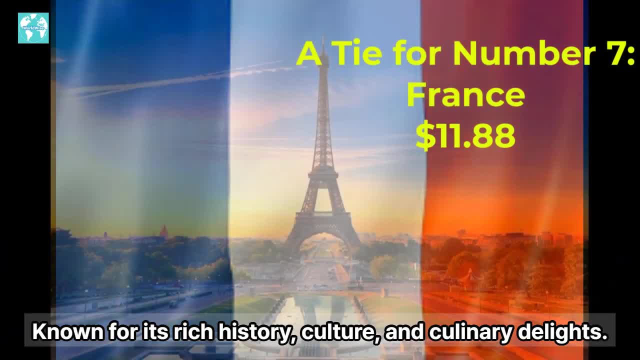 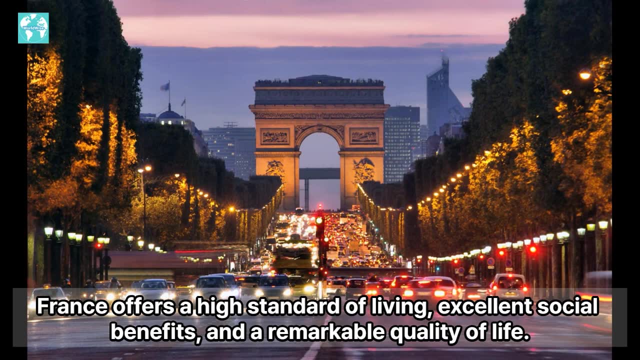 A tie for number 7.. France: Known for its rich history, culture and culinary delights, France offers a high standard of living, excellent social benefits and a remarkable quality of life. Working in sectors such as finance, technology or hospitality in France. 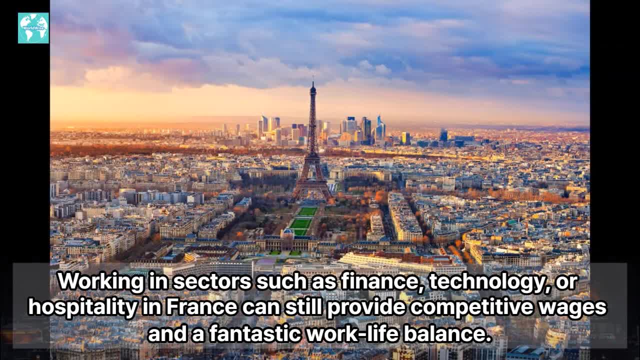 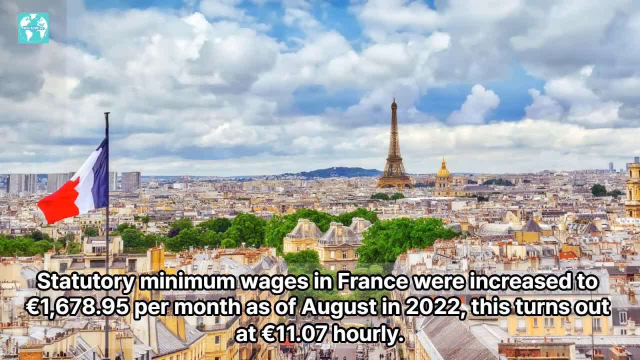 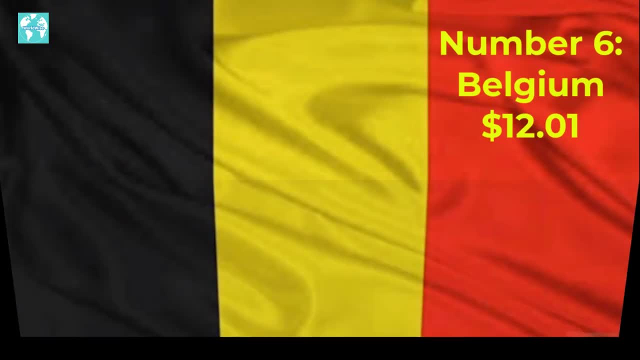 can still provide competitive wages and a fantastic work-life balance. Statutory minimum wages in France were increased to €1,678.95 per month as of August in 2022.. This turns out at €11.07 hourly. Number 6. Belgium, With its highly 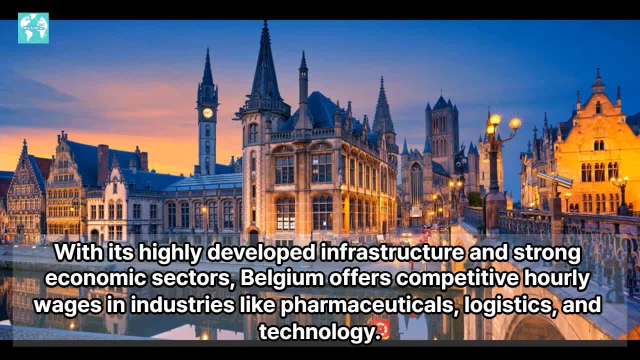 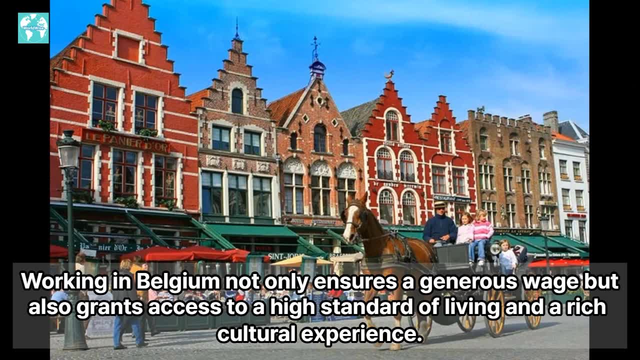 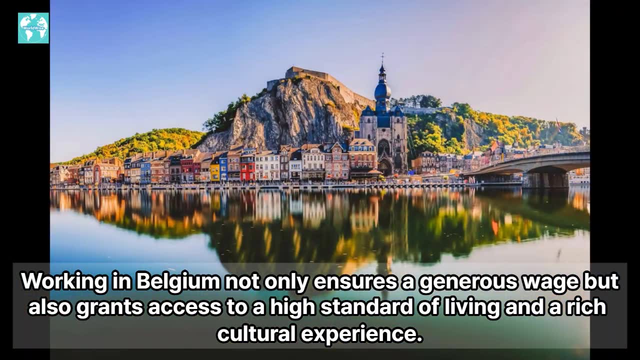 developed infrastructure and strong economic sectors. Belgium offers competitive hourly wages in industries like pharmaceuticals, logistics and technology. Working in Belgium not only ensures a generous wage, but also grants access to a high standard of living and a rich cultural experience. As of April 1, 2022, the minimum wage equals €1,842.28. 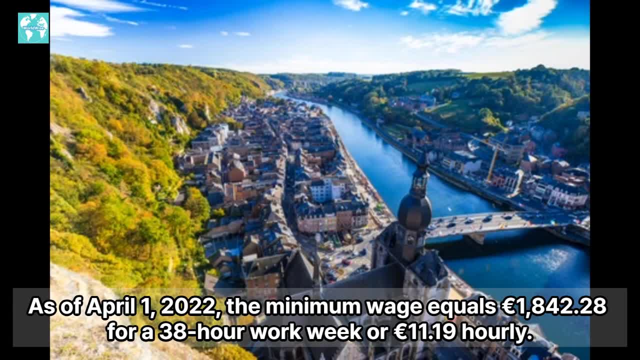 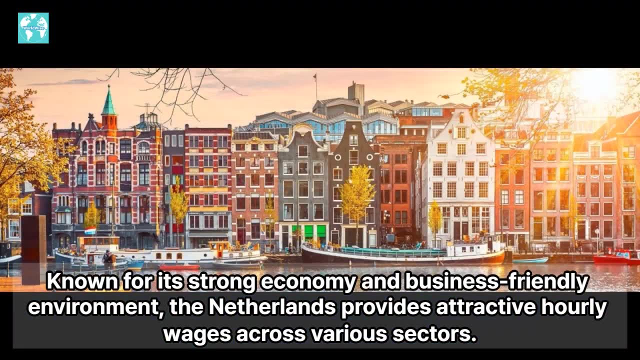 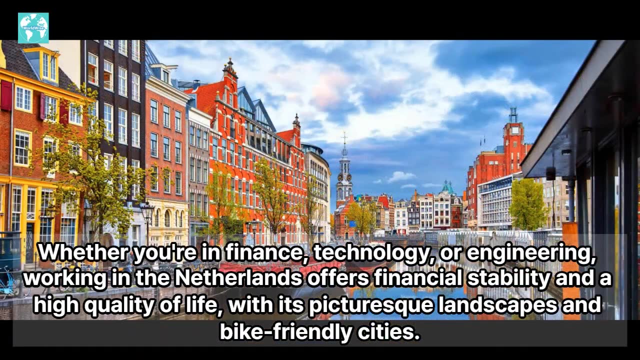 for a 38-hour work week or €11.19 hourly. Number 5.. Netherlands: Known for its strong economy and business-friendly environment, the Netherlands provides attractive hourly wages across various sectors, Whether you're in finance, technology or engineering, working in the Netherlands. 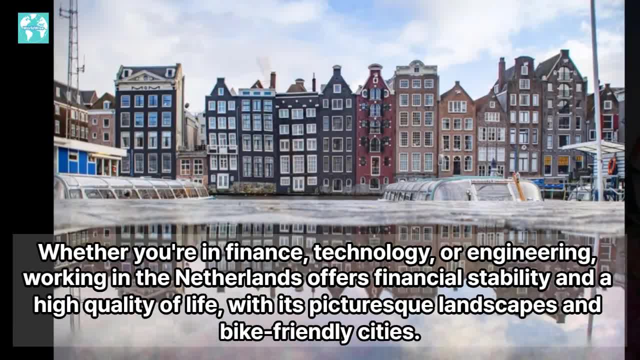 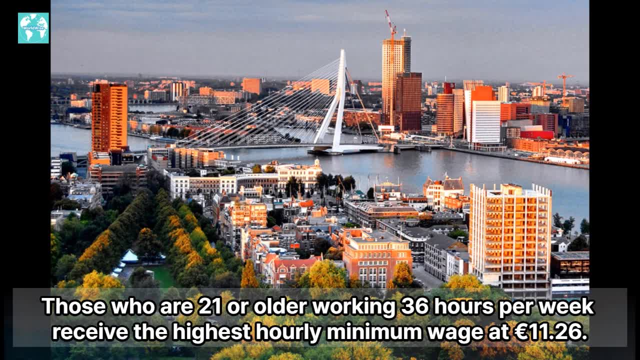 offers financial stability and a high quality of life, with its picturesque landscapes and bike-friendly cities. Those who are 21 or older, working 36 hours per week, receive the highest hourly minimum wage at €11.26.. Number 4. New Zealand. 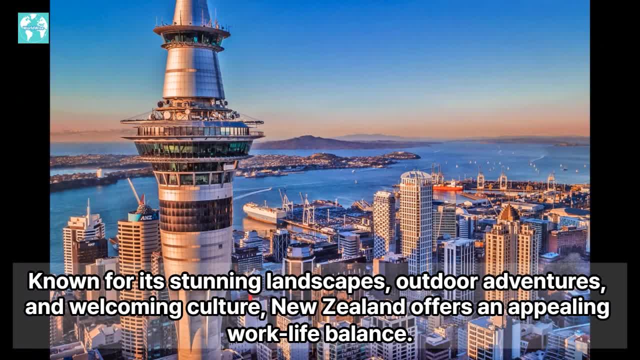 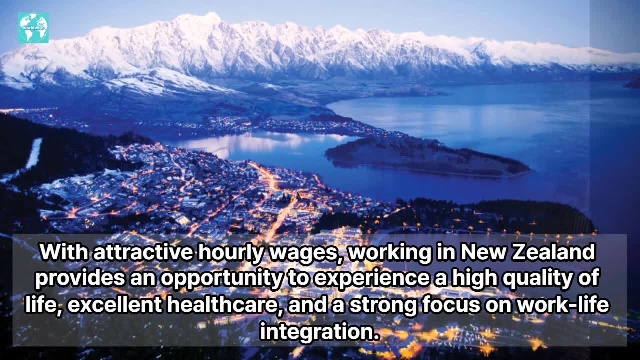 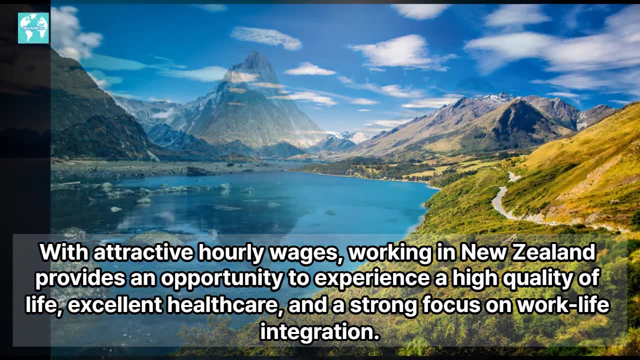 Known for its stunning landscapes, outdoor adventures and welcoming culture. New Zealand offers an appealing work-life balance With attractive hourly wages. working in New Zealand provides an opportunity to experience a high quality of life, excellent health care and a strong focus on work-life integration. 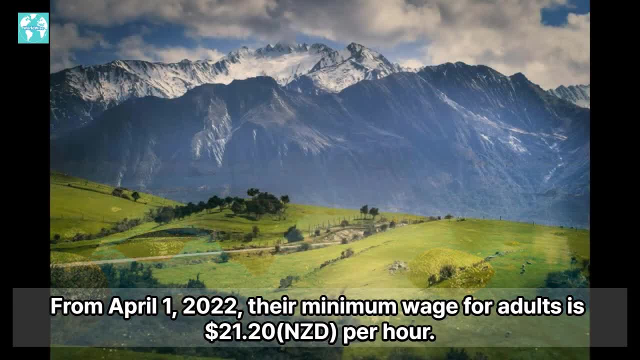 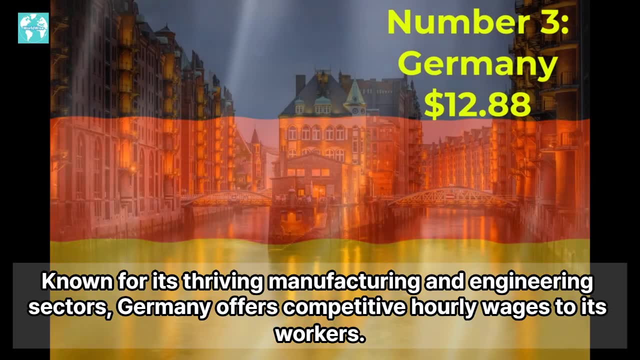 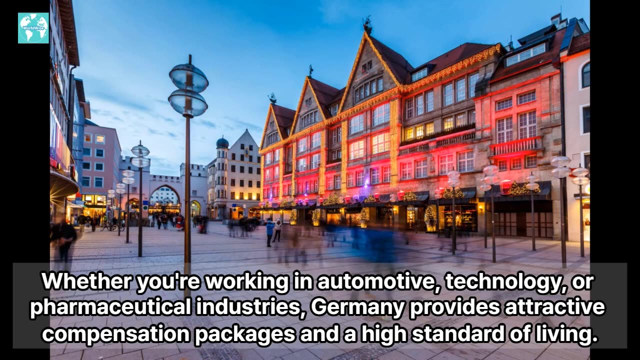 From April 1, 2022, their minimum wage for adults is $21.20 per hour. Number 3. Germany, Known for its thriving manufacturing and engineering sectors, Germany offers competitive hourly wages to its workers, Whether you're working in automotive technology or pharmaceutical industries. 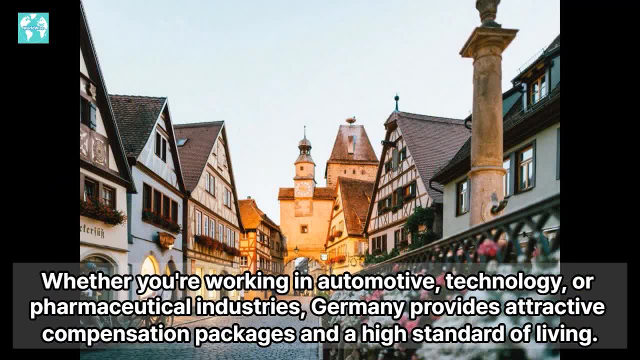 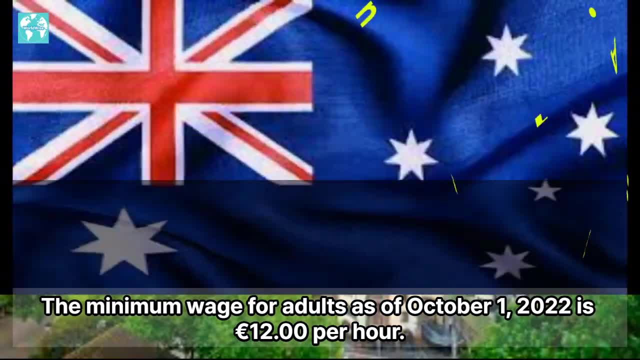 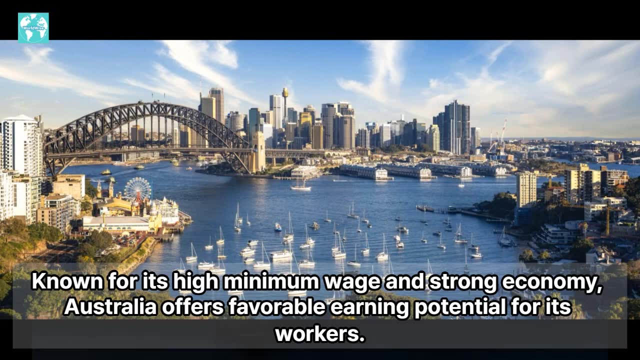 Germany provides attractive compensation packages and a high standard of living. The minimum wage for adults as of October 1, 2022, is €12 per hour. Number 2.: Australia: Known for its high minimum wage and strong economy, Australia offers favorable earning potential for its workers. 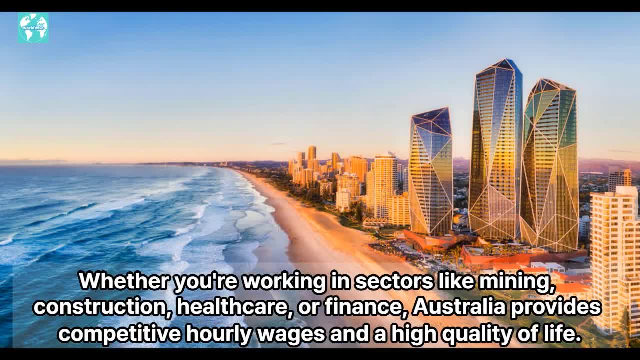 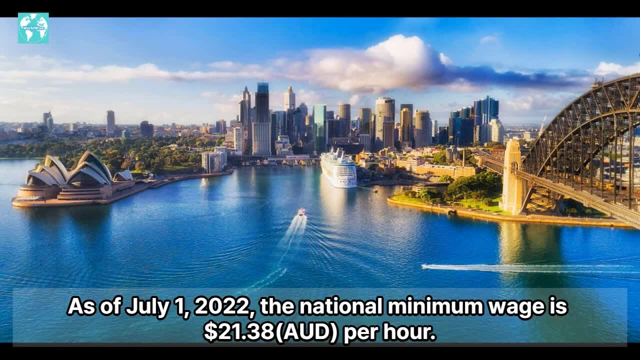 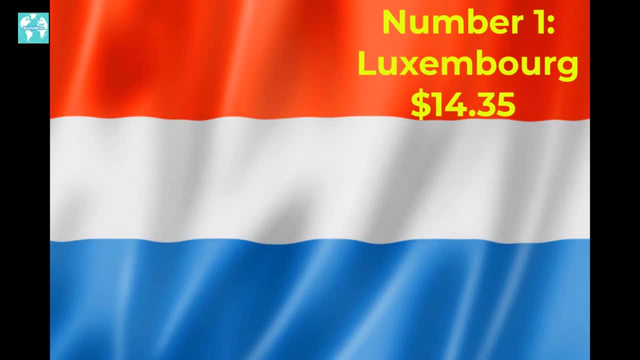 Working in sectors like mining, construction, health care or finance. Australia provides competitive hourly wages and a high quality of life. As of July 1, 2022, the national minimum wage is $21.38 per hour. Number 1. Luxembourg, Known for its wealth and financial services sector. 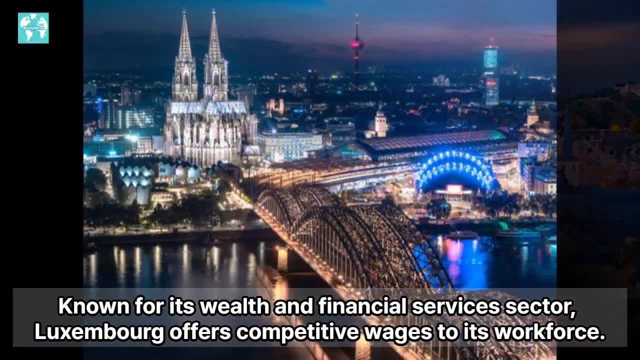 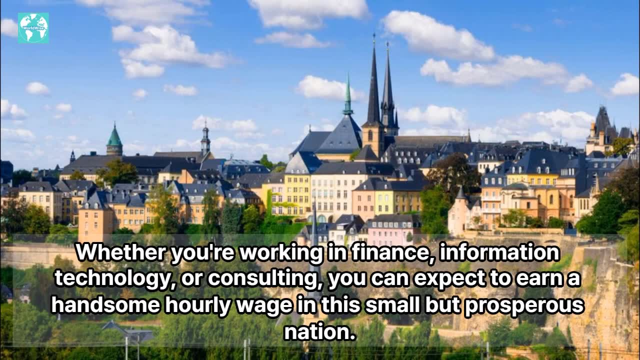 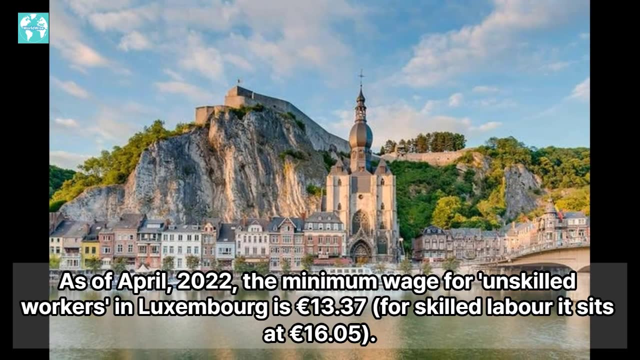 Luxembourg offers competitive wages to its workforce. Whether you're working in finance, information technology or consulting, you can expect to earn a handsome hourly wage in this small but prosperous nation. As of April 2022, the minimum wage for in Luxembourg is €13.37,. 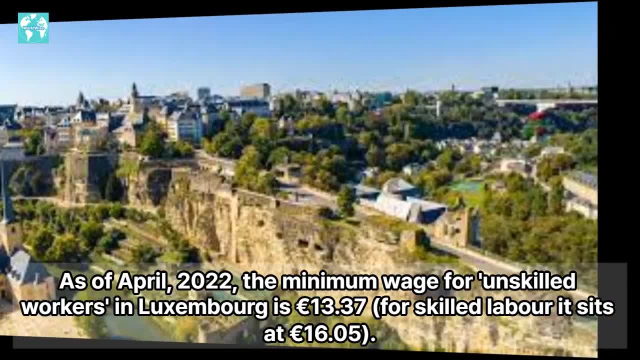 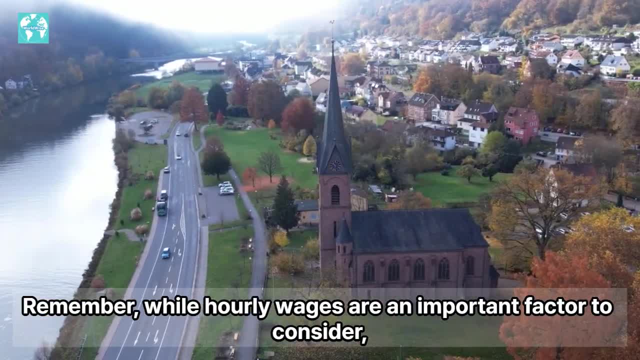 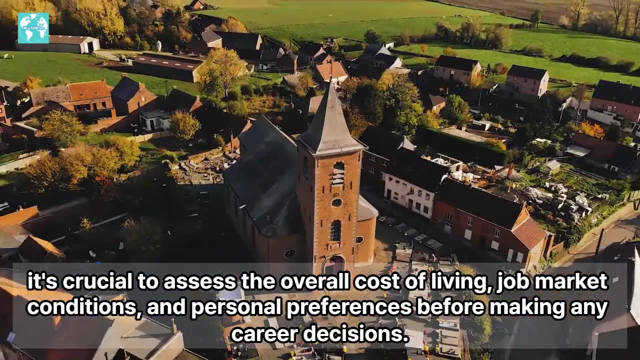 for skilled labor, it sits at €16.05.. And there you have it, our list of the top 10 countries with the highest hourly wages. Remember, while hourly wages are an important factor to consider, it's crucial to assess the overall cost of living, job market conditions and personal preference. 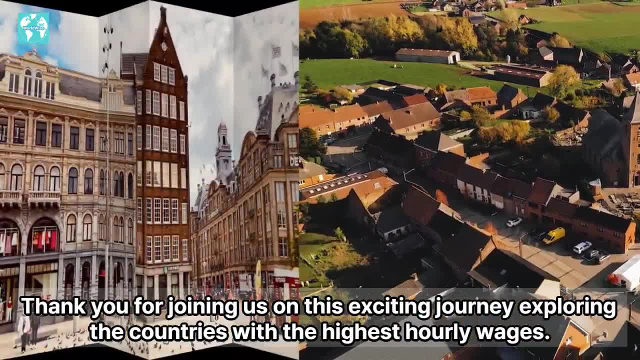 If you want to learn more about the top 10 countries with the highest hourly wages, you can check out our video on the top 10 countries with the highest hourly wages. If you found this video informative and enjoyable, don't forget to like.